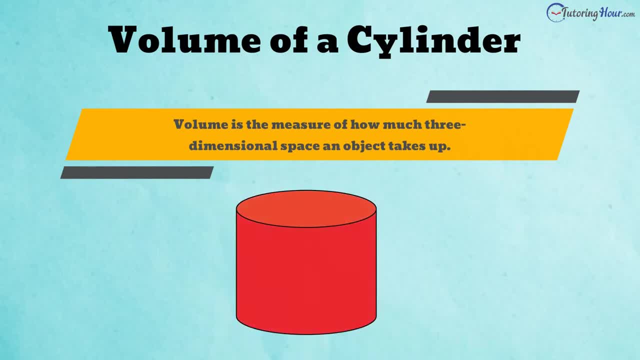 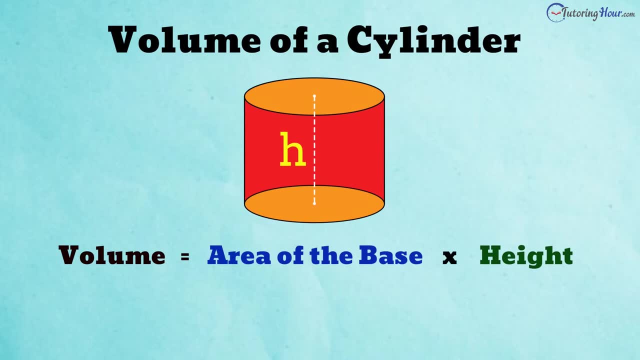 measure of how much three-dimensional space an object takes up, and the volume of a cylinder is calculated by multiplying the area of the base of the cylinder with its height. Take a look at this cylinder. It has a circular base. The area of a circular base is pi times r. 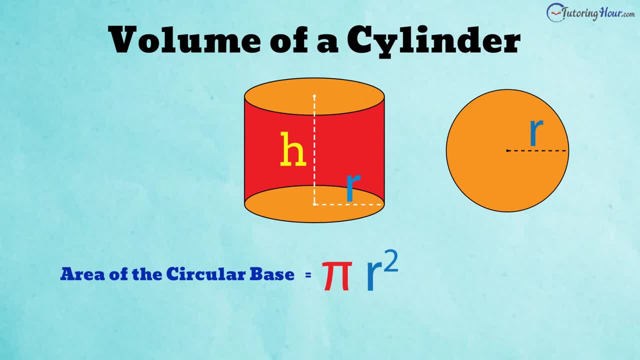 squared where r is the radius of the base. Now, volume is equal to area of the base times the height of the cylinder, and that is pi times r, squared times h. Let's apply the formula to find the volume of this cylindrical candle: The height of the candle. 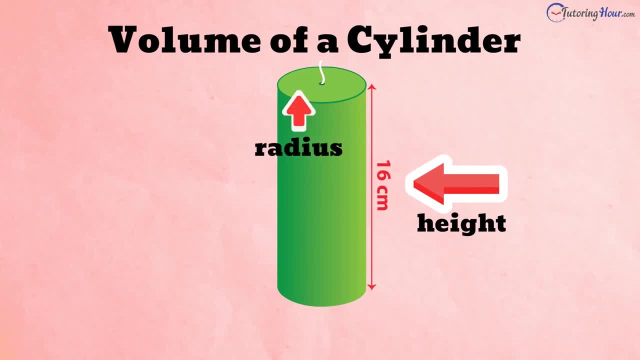 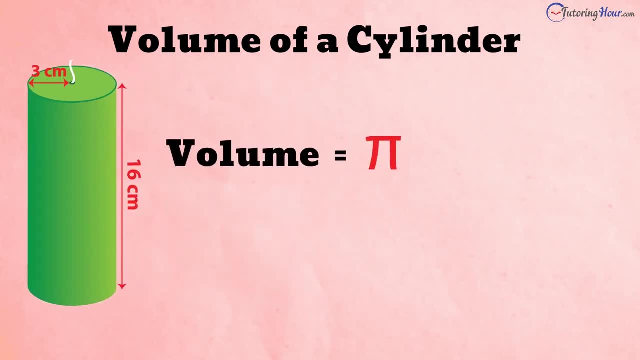 is 16 centimeters and the radius of its base is 3 centimeters. Let's write the formula: Volume is equal to pi times r squared times the height of the cylinder. Plugging the values we have: pi times 3 centimeters squared times 16 centimeters, which is pi times 9 centimeters squared times 16. 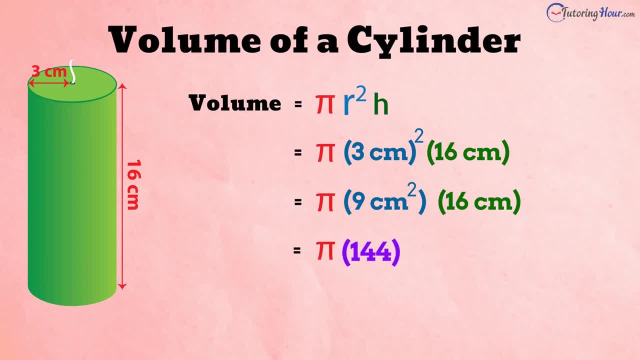 kilometers. So volume is equal to pi times 16 centimeters squared times 16 centimeters P of party square root of standard, whereas it is pi times a hundred hundred percent square ofcale моя, which makes the volume pi times 144 cm³, which can also be written as 144. luxurious su hinter holding. 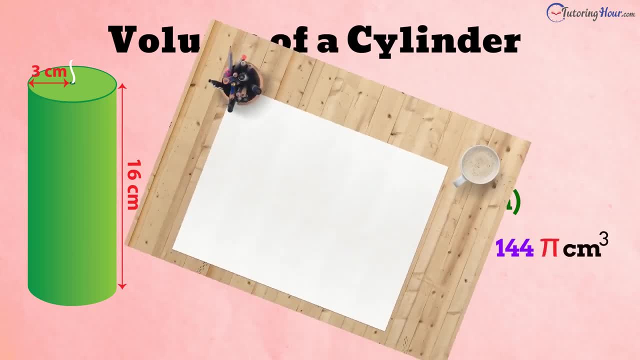 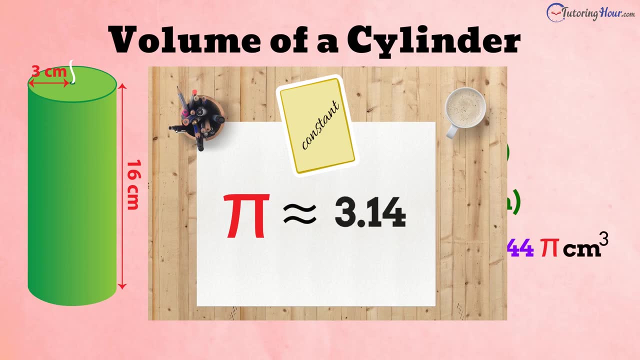 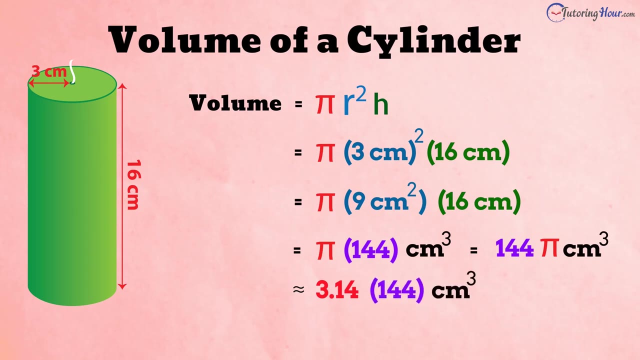 pi cubic centimeters. We could stop here or go ahead and substitute the value of pi, which is a constant, and its value is approximately 3.14.. We will find the product of 3.14 and 144 cm³. The volume of the candle, therefore, is US***4.. conveying the regular value of the concentration of 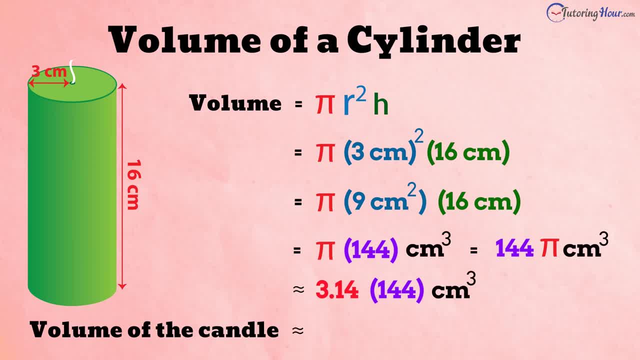 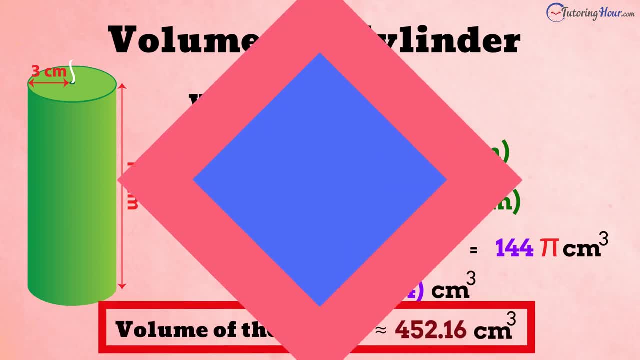 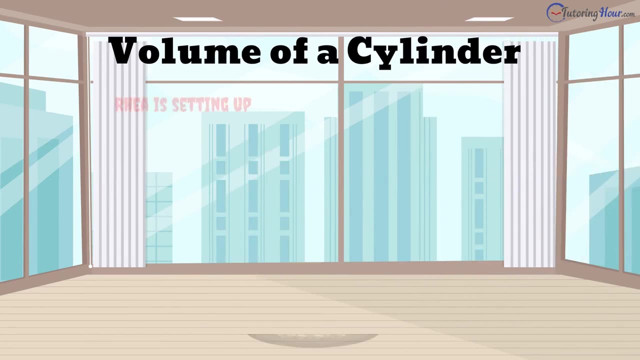 mayonnaise above the hot temperature at 40° C. that holds the volume up to using. volumgence स is approximately 452.16 cubic centimeters. Let's understand finding the volume of cylinders better with this scenario. Raya is setting up a cylindrical aquarium at her home. 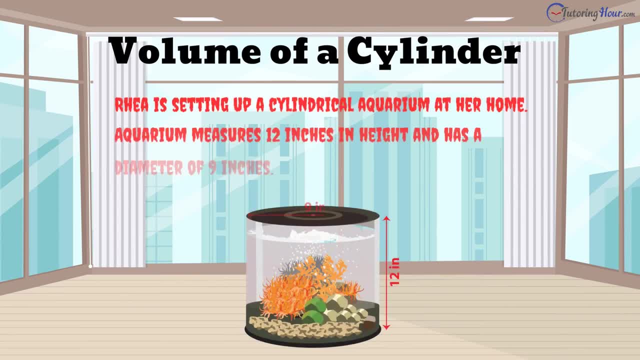 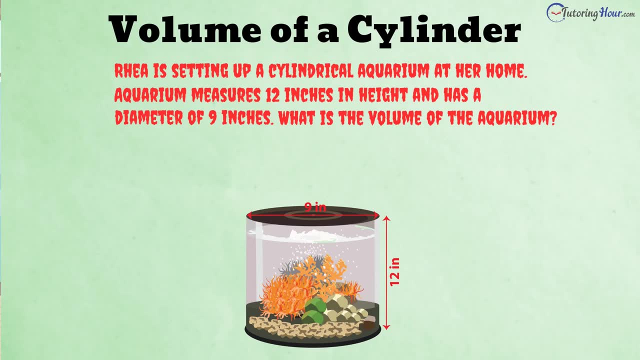 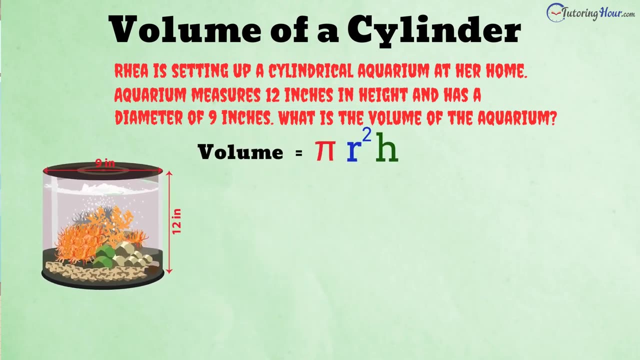 The aquarium measures 12 inches in height and has a diameter of nine inches. What is the volume of the aquarium? First, let's see what information we have. We have the diameter and the height. Let's write the formula for finding the volume of cylinders.